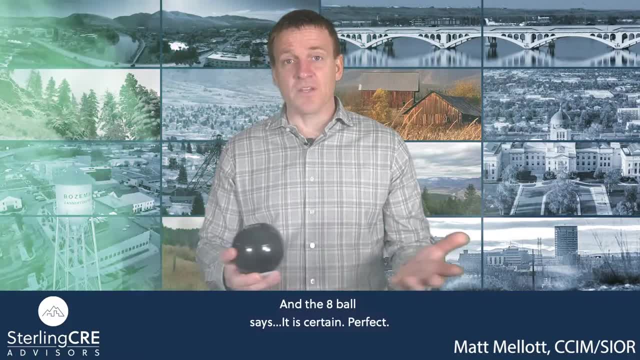 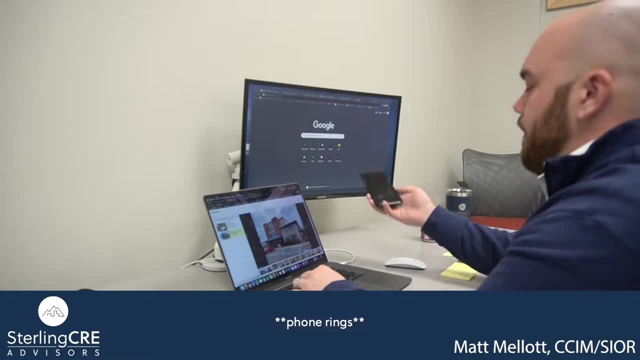 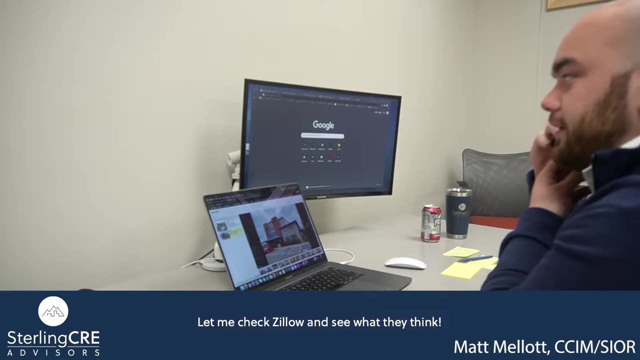 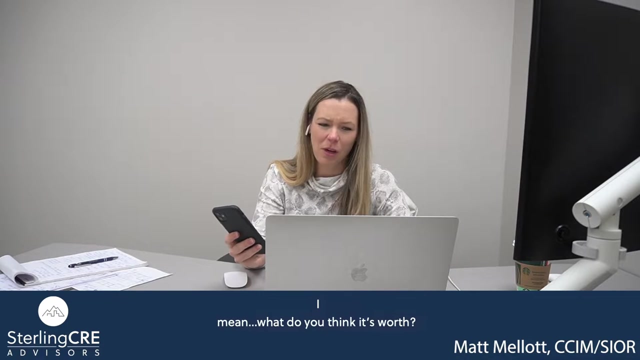 did, I guess, the right price And the 8 Ball says it is certain. Hello, this is Nick. Oh, yeah, okay, I know what you're talking about. Let me check Zillow, see what they think. One second here. Well, what do you think it's worth? Okay, that sounds good. 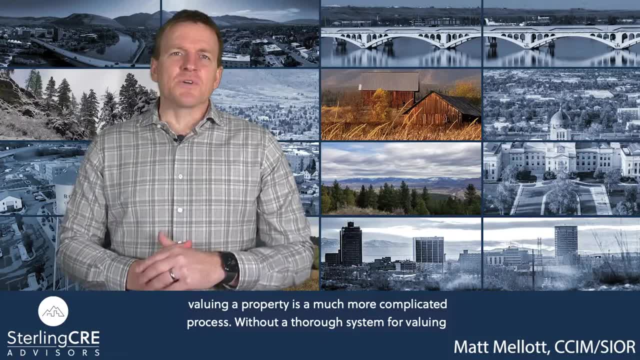 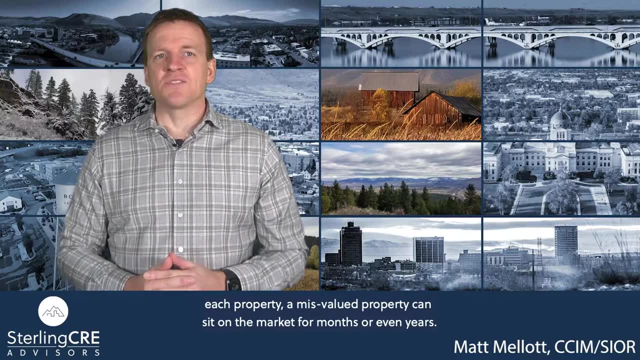 We are, of course, just kidding. In fact, valuing a property is a much more complicated process. Without a thorough system for establishing value, a misvalued property can sit on the market for months or even years When clients come to us to determine the value of their building. 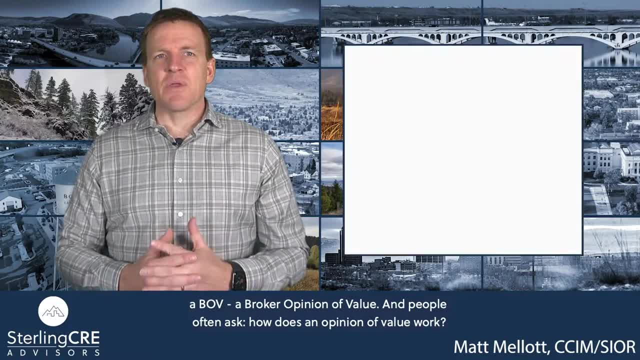 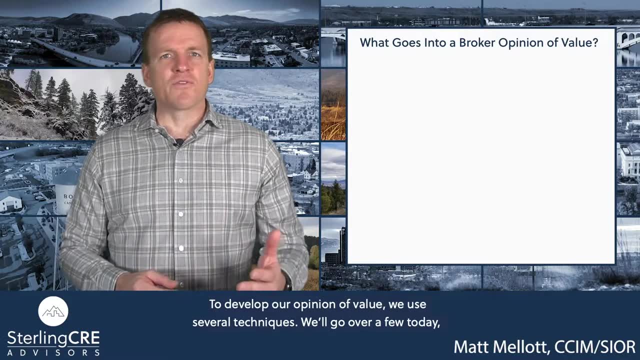 we produce a BOV, a broker opinion of value, And people often ask: how does an opinion of value work? To develop our opinion of value, we use several techniques. We'll go over a few today, but this is a very general overview. Every property evaluation is developed with a. 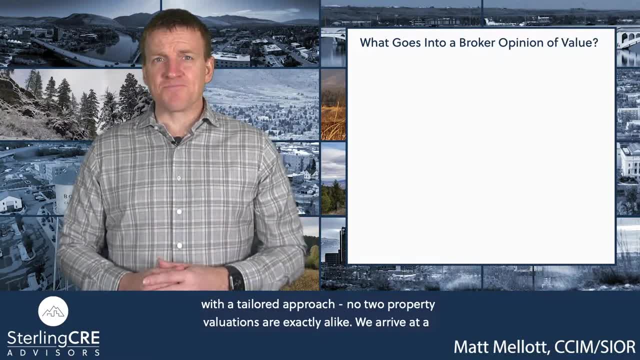 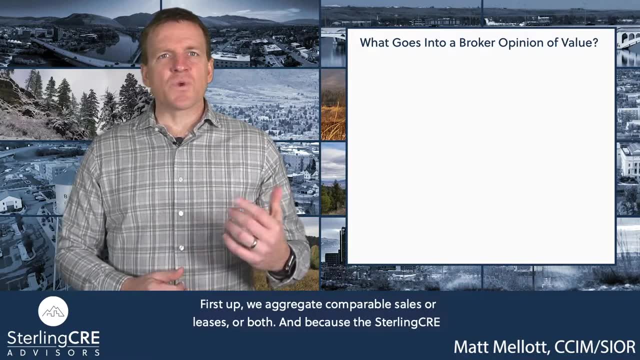 tailored approach. No two property valuations are exactly alike. We arrive at a value that is based in local data, national best practices and considers regional market factors. First, we aggregate comparable sales or leases or both, And because the Sterling CRE team maintains the 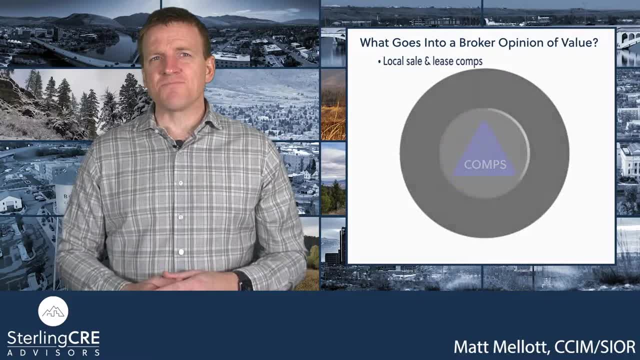 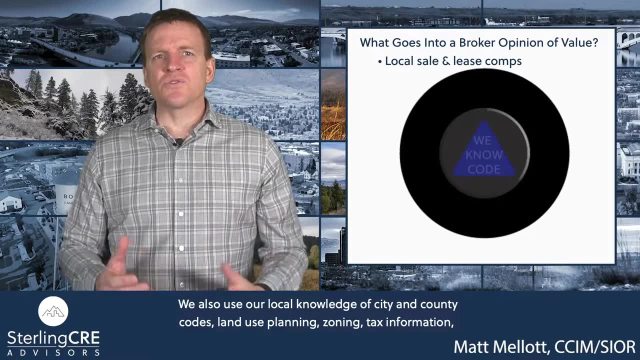 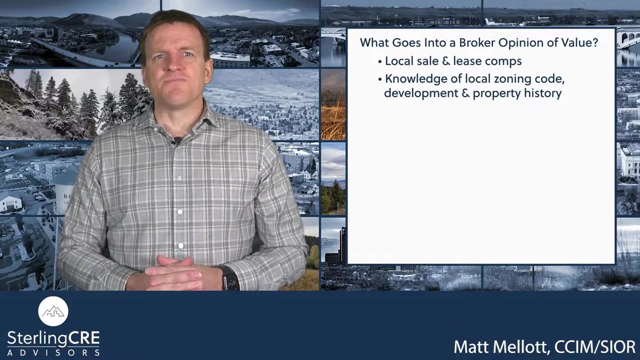 largest private proprietary library of local commercial sales data. we have the most accurate sales and leasing information that's available. We also use local knowledge of city and county codes, land use planning, zoning, tax information and building features or bugs to provide additional context for evaluation range. But comps aren't the only way to evaluate. There are 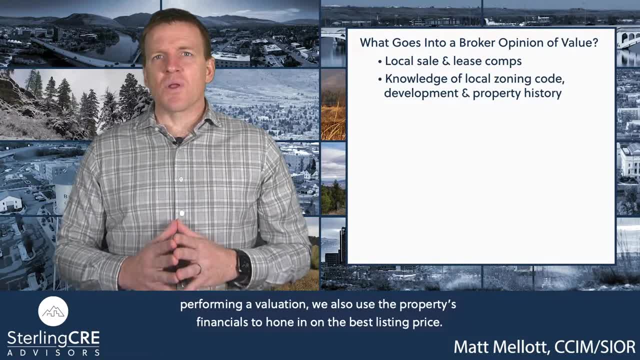 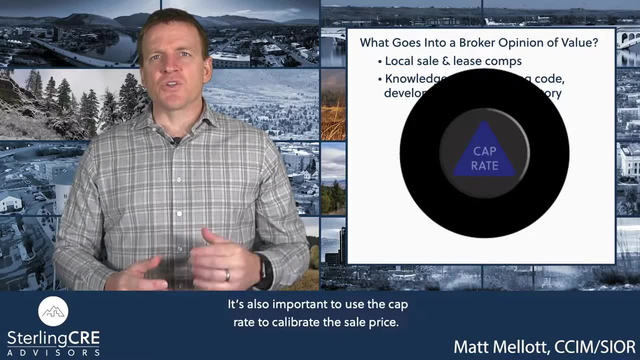 many ways to understand the most accurate valuation. When performing evaluation, we also use the property's financials, when applicable, to hone in on the best listing price. It's also important to use a cap rate to calibrate the sales price. A capitalization rate is one way. 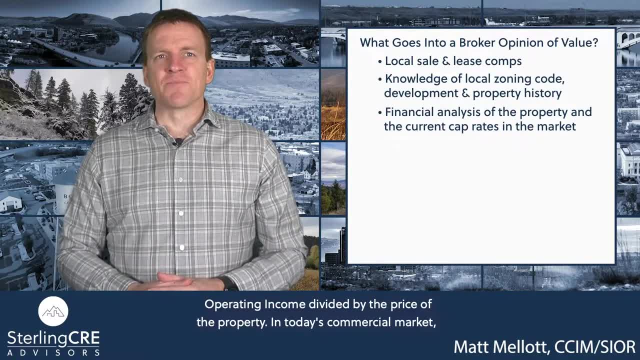 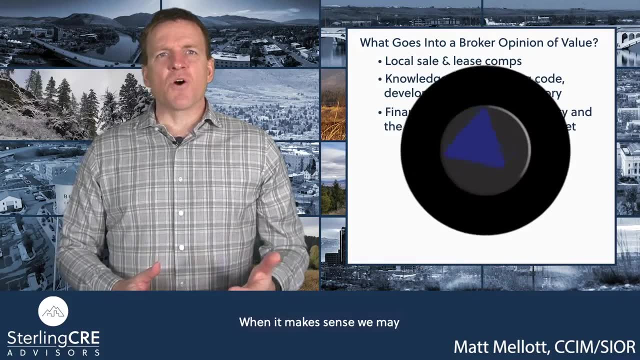 to evaluate the investment performance of a given property In today's commercial market. most cap rates we see fall in the five to eight percent range, depending on asset type. When it makes sense to do so, we'll also run discounted cash flow analysis to determine a given property's.